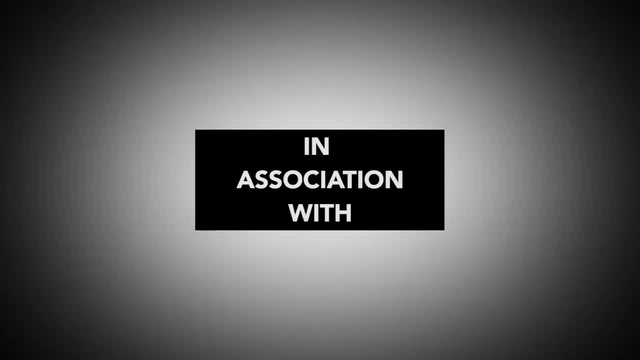 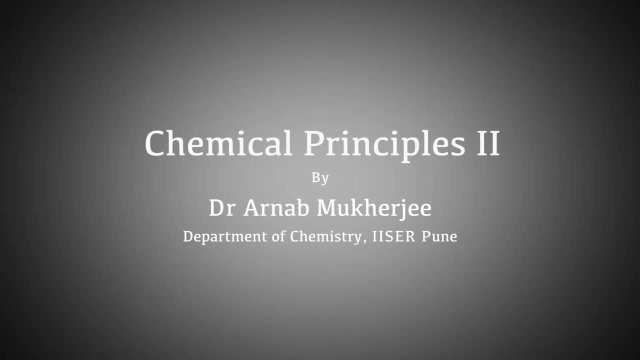 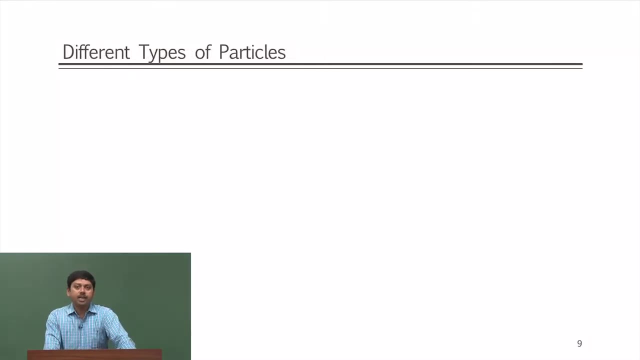 Now, what will happen if the particles were indistinguishable And what is the situation? what are the situation in which indistinguishable particle arise? So, as I said, the classical particles are distinguishable because each particle follows a particular trajectory. therefore, you can detect the particle even when they are close together, because the 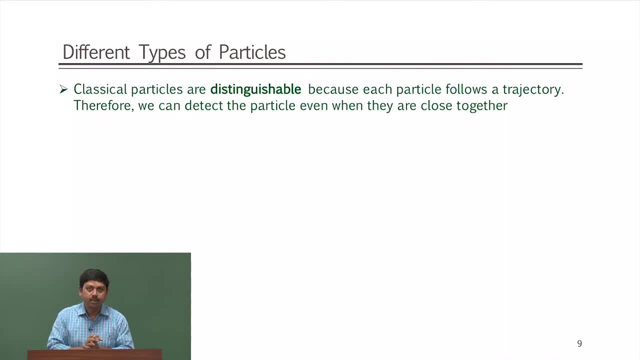 classical particles really will not like collapse on to each other. you know you can still there will be particles, even if they are come closer. you can still say this is particle 1, this is particle 2, because we have been following that particle all along. However, for quantum, 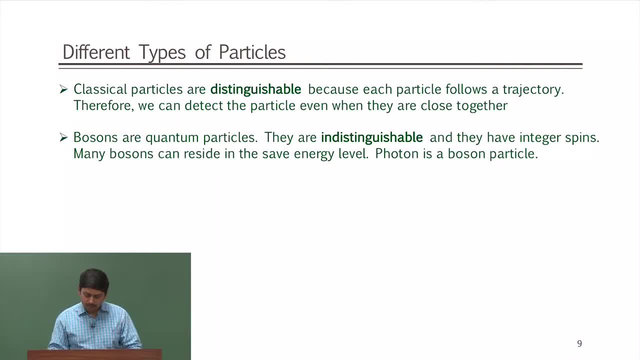 particle, for example bosons and fermions. they are indistinguishable. so, bosons, there are two kinds of quantum particles are there, one is called boson, which are, you know, those are indistinguishable and they have, you know, integral spins, another characteristics of 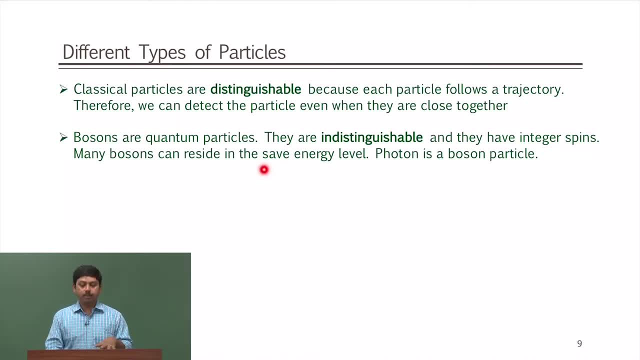 boson is that many of the bosons can decide on the same energy level. so photon is a boson particle, like Higgs boson. people know about a lot that is a you know boson. that is a that has integral spins. Similarly, electron protons also are indistinguishable. they are quantum particles. the reason they 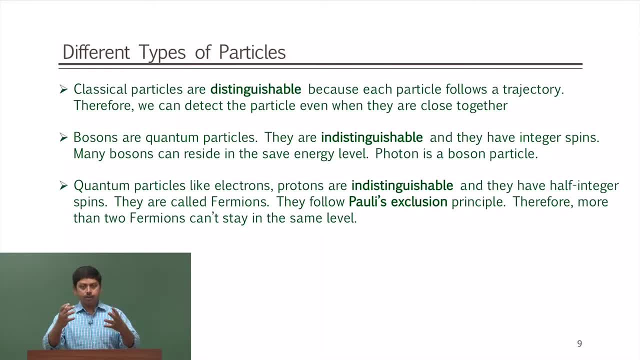 are indistinguishable is that when you know- let us say you know- hydrogen molecule, when two electron come close together and form bond, you can never distinguish which is electron 1 and electron 2, all that you write is a wave function associated with both the electrons. 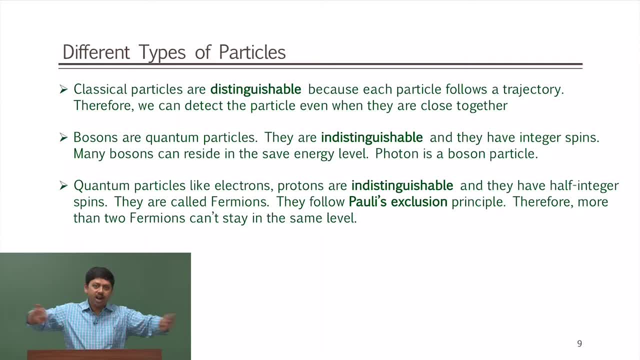 together you do not identify. So when they are far apart, maybe You know, hydrogen atom has electron 1, hydrogen atom number 2 has electron 2, but when they are close, then you cannot distinguish the electron anymore. So therefore electrons are indistinguishable particles and they are fermions because they 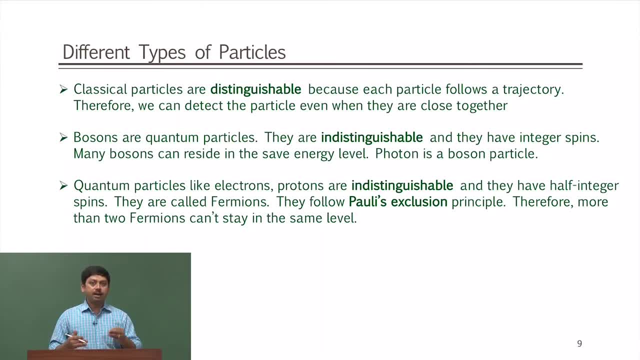 have half integer spins and fermions have a speciality that not more than two fermions can stay in the same energy level due to PauliÕs exclusion principle. So for fermions the energy level can have either 0,, 1 or 2 particles. 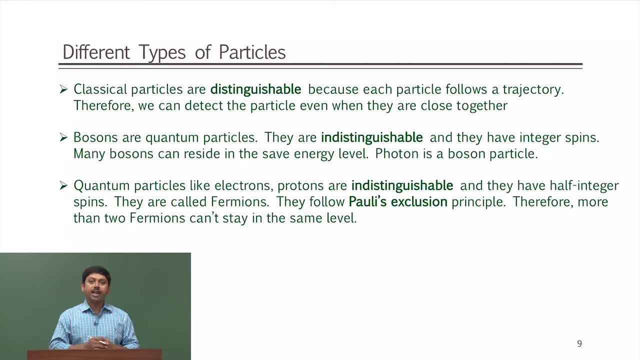 For bosons, however, you can have any number of particles. however, both fermions and bosons are indistinguishable particles, unlike classical one, which are distinguishable particles. So in that case, then, we have to still identify how to get the statistics, how to calculate, 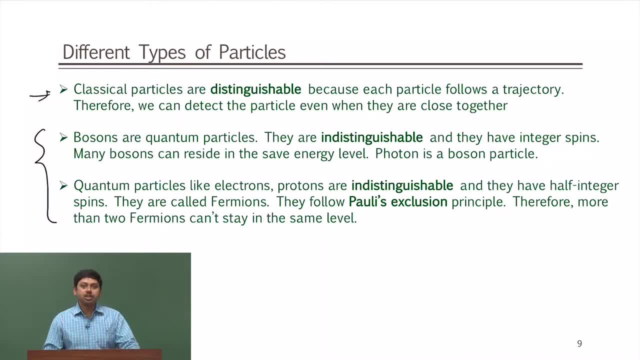 WÕs and how to get you know the distributions, or probability distributions, of the particles in different energy levels with respect to the energy. So let us see that. So we will see that bosons and fermions will follow different statistics, and this is called. 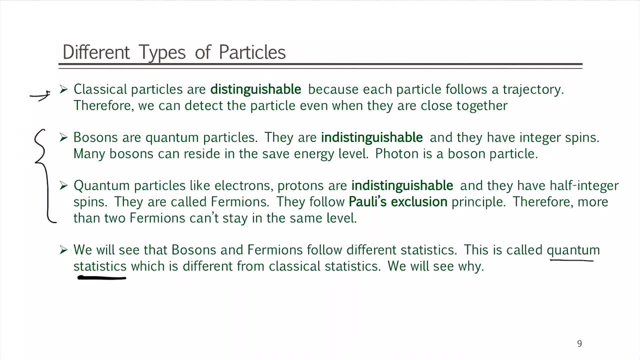 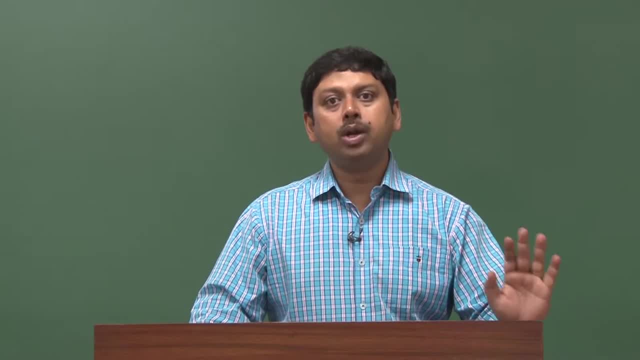 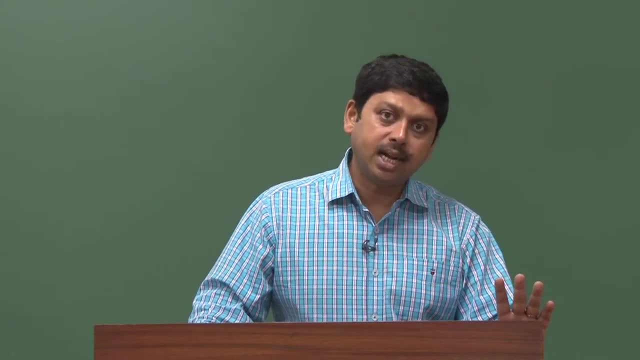 quantum statistics. It may be, you know, you know- intimidating for you to knowing the term quantum statistics, but in this particular course we are not going to go into mathematical detail of derivations of any of those quantum statistical formula. All that we are emphasizing at this point is that these particles are indistinguishable. Rest of the things are. 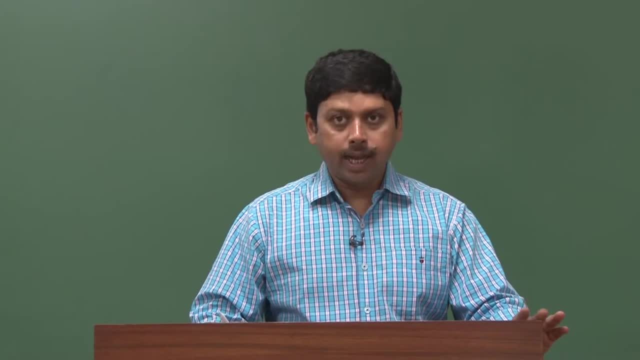 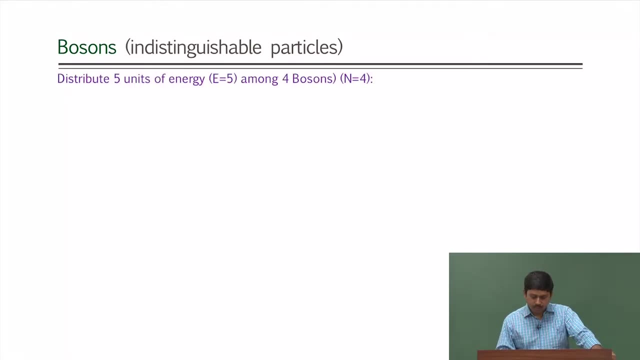 same as what we have discussed. 1, So it will not be complicated, as you can see soon. So let us talk about bosons. Again, we are going to talk about the same thing: 5 units of energy, 4 particles, Only thing, the. 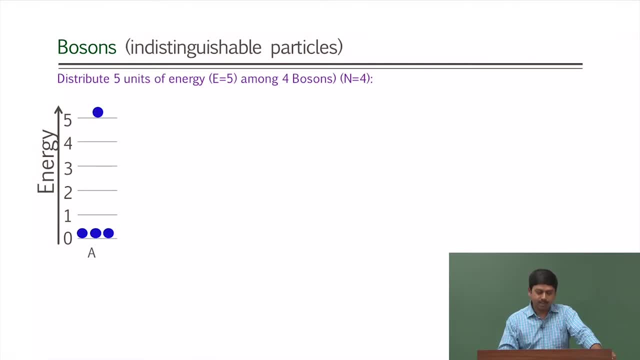 picture will look very different. now. The picture will look like this: all are blue particles. Remember the earlier ones where they had different colors, So colors were distinguishing the particles for us basically. So now we are putting all same color. so, for example, we will say the green particle is a green particle, It is the color of the 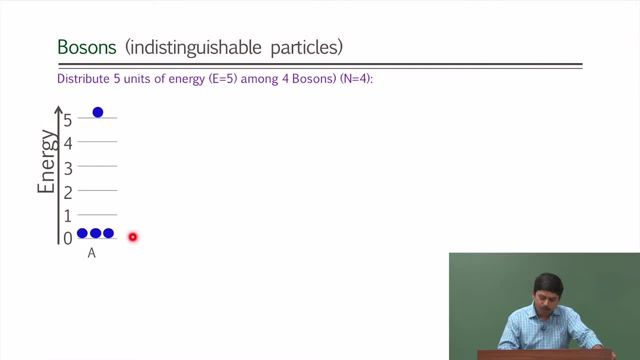 green particle. So now we are putting some colors. We will not looking at the colors as if, but a lot of colors. Life of the particles is going to be different, so let us not think a lot about it because there are so many color colors actually. 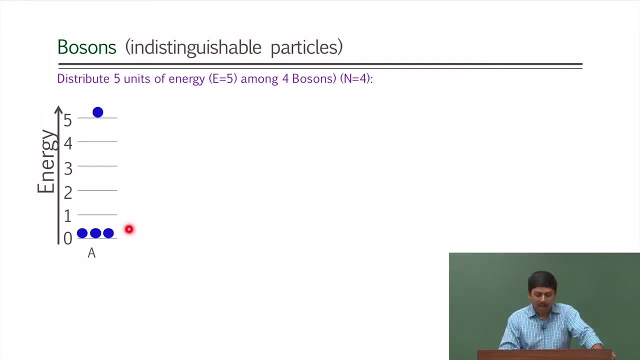 So therefore, we can no longer distinguish whether the green particle is up or red particle is up, or which particle is up. So how many possible ways we can get this distribution? Only one possible way, because either we bring, whatever particle we bring, we do not know. 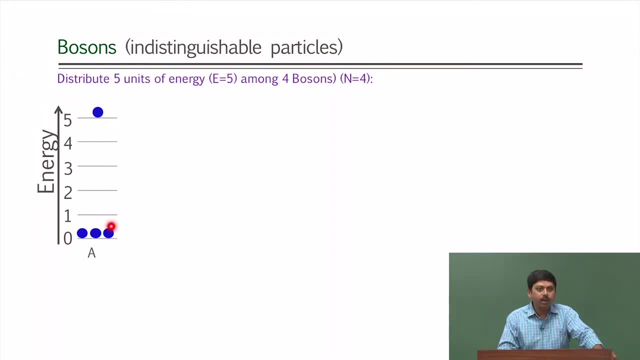 which particle we are bringing up right. So there can be only one way of getting so. the number of micro states for distribution A is 1.. Remember, however, the number of distribution still remains to be p in 4.. Partition of 5 units of energy in to 4 particle. 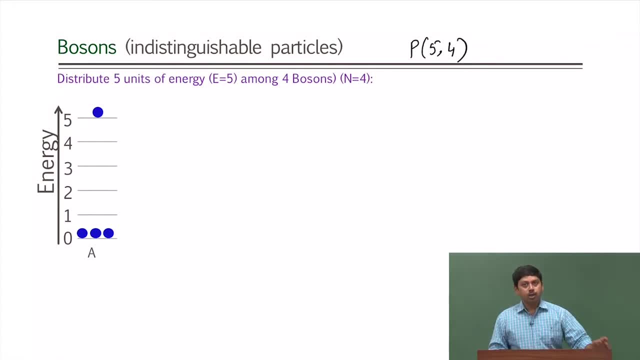 Viewers, how many micro states can we get from 1 by A, 5 units of energy into 4 particle, so P54 will be still 6,. however, individual microstates of individual distribution will be just 1 instead of N. factorial by N1. factorial N2. 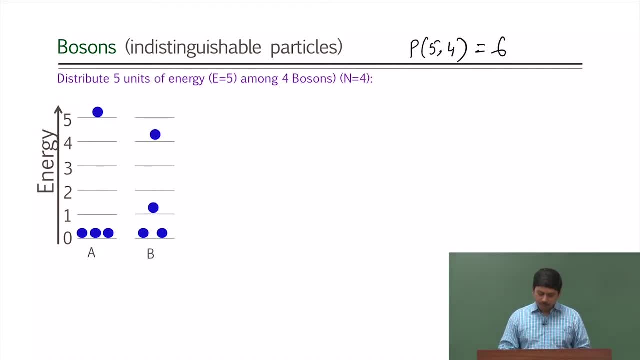 factorial, because this is no longer distinguishable. so these are the 6 possible distributions that we had shown you before. but only thing is that in that particular case you had all different colours. now you have all same colour and because of that all the Ws now are 1,. 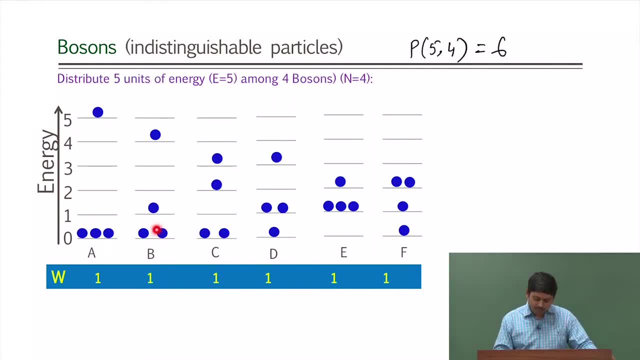 you can no longer distinguish that, whether which particle has gone up and which gone down. So then, automatically, what we get is that we get 6 distributions and we got only 6 microstates. remember how many? we got 56 microstates, we got all total when the particles were distinguishable. 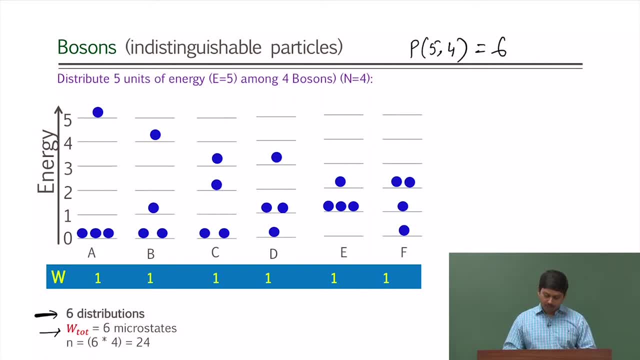 now with indistinguishable particles, we only get 6 possible microstates. Okay, So number of particles in all 6 possible microstates is 4 into 6 is 24, so total, there are 24 dots in this graph. and now we want to identify how many particles are there in which level. 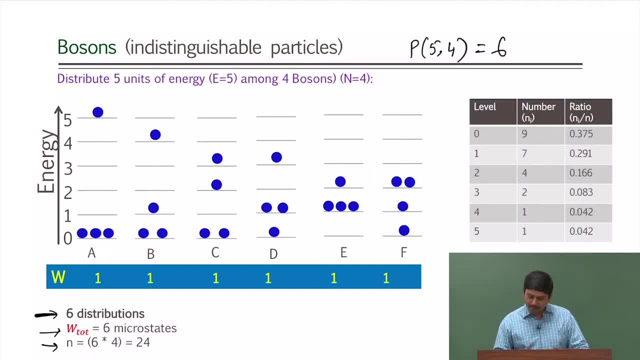 so, for example, you see that level 1 has 5 particles. sorry, energy level 5 has 1 particle. energy level 4 also has only 1 particle. energy level 3 has 2 particle. now we have only 1,. 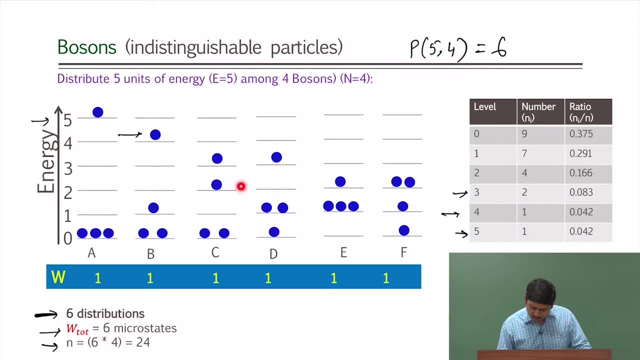 this 1 and this 1, energy level 2 has 4 particle, energy level 1 has 1,, 2,, 3,, 4,, 5,, 6, 7 particle and energy level 0 has 3 plus 2, 5 plus 2,, 7,, 8, 9 particles. 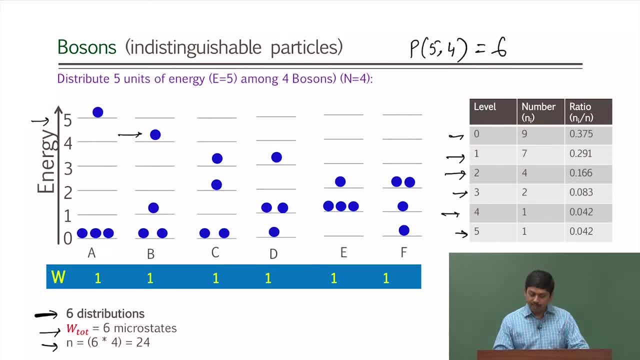 So you see, each energy level. we can just count from this distribution and we can get the number of particles in each energy level. and now, since we are combining all possibilities, then we are dividing. we have to divide this 9 by 24 to get 24.. 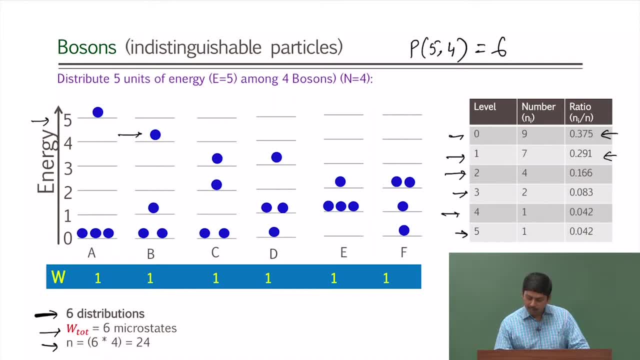 Okay, Okay. And then we have to get the n? i by n. so this is the probabilities, n? i by n, as is shown here for each energy level. So now, the same way we similarly what we got for distinguishable particles for bosons. 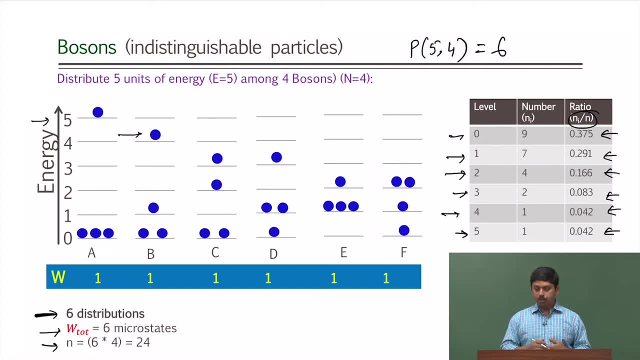 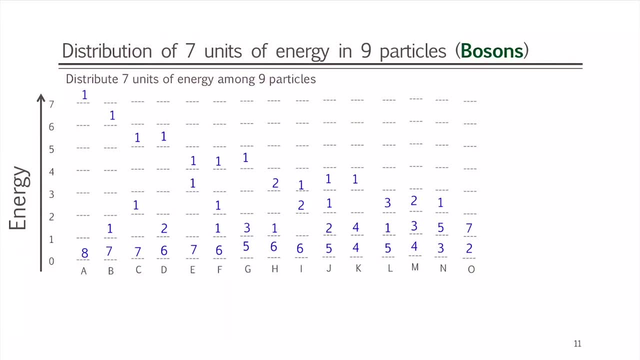 we get the same thing. we get the similar distributions for bosons also, and that is given by these numbers and we can plot them. before we do that, let us assume for 7 units energy, 9 particles. in this particular case also, the number of distributions will be same. 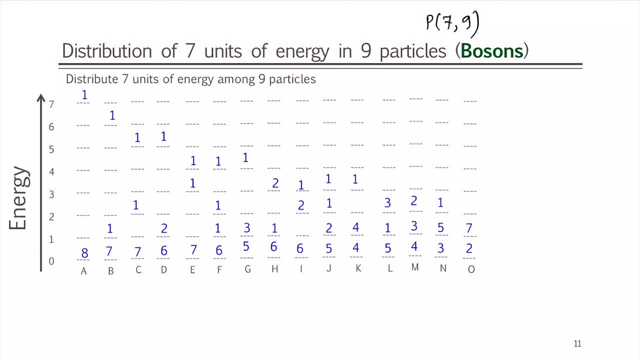 as 15, which we had before, which is obtained from partition of 7 into 9.. And here also we have similar distributions like A, B, C, D. however, here also the number of microstates for each of the distribution will be just 1, because particles are distinguishable. 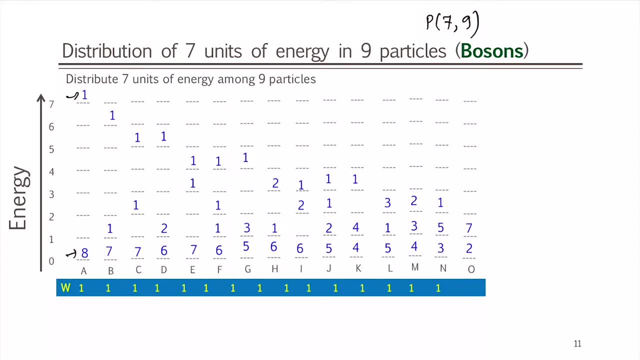 Note that we have not put with dots because there is not enough space for putting 8 dots here. but this 8 denotes just 8 blue particle and this denotes just 1 blue particle. For example, here it denotes 7 blue particle, 1 blue particle, 1 blue particle, so just. 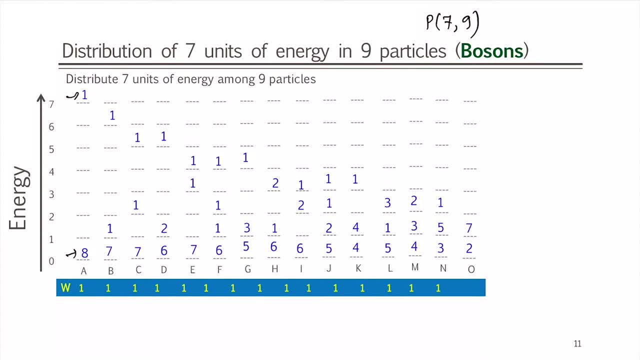 imagine that they are all blue. So earlier we did N factorial by N1 factorial and all that. here we cannot do that because they are all distinguishable. indistinguishable, therefore, they are all just 1.. Now, once you get that, how many microstates? 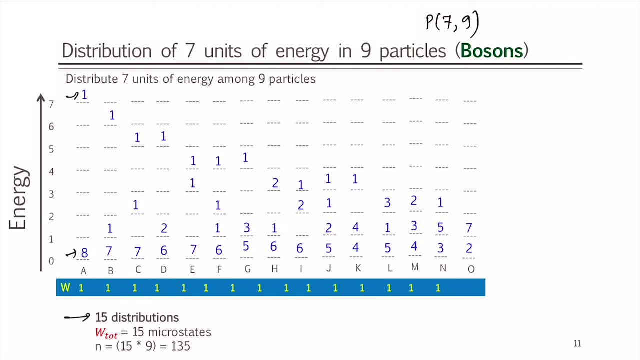 Then. so 15 distributions. each distribution give you 1 microstate, so W tot is just 15.. So total number of particles from all possible distribution is 15 into 9, because we have only 9 particles and 15 distributions. 15 into 9 is 135. 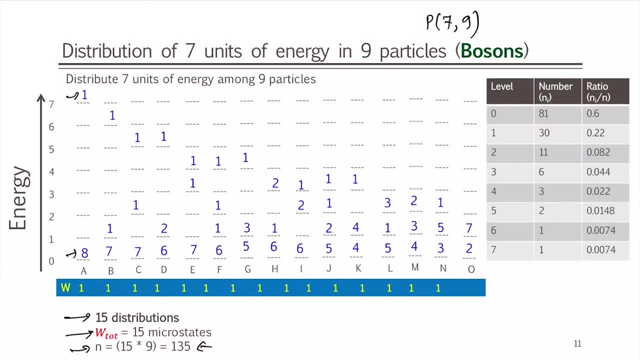 Now we can count how many particles are there, in which level. let us start with 7,. 7 has only 1 particle, so 1 particle. now probability is 1 by 135, which is given by this number. Level 6 has 1 particle. 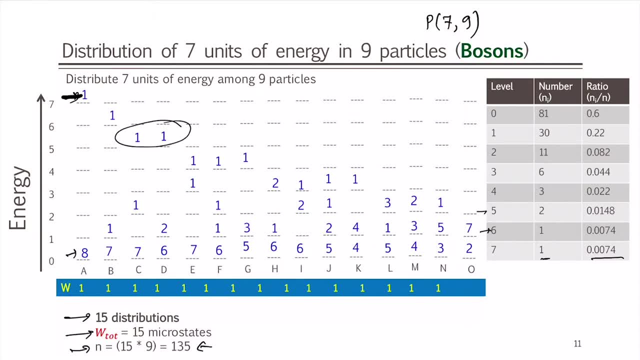 Level 5 has 2 particle, as you can see from this. level 4 has 3 particle, as you can see from this, and level 3 has 1 plus 2, 3 plus 3, 6 particle, as you can see from here level. 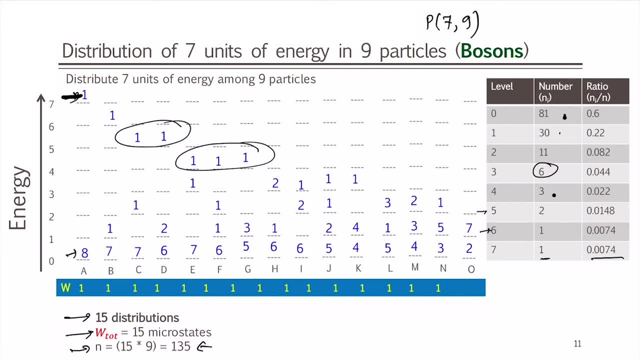 2 has 11, level 1 has 30 and level 0 has 81, you can count that, You know. if you do not want to count, then there is an easier way to do. that is when you partition 7 into 9.. 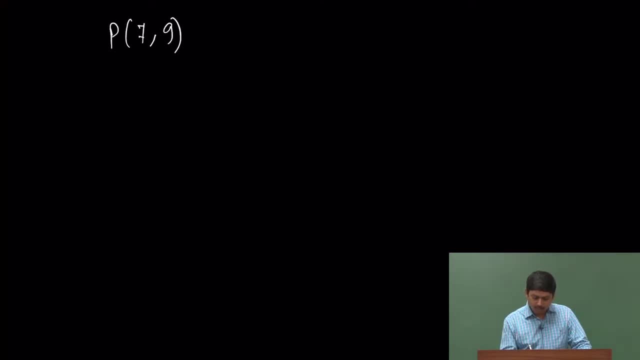 So you can do that, So you can do that, So you can do that, You can do that, You can do that, So you can do that, So you can do that, Which I will just show you one or two examples. let us say you partition 7 into 9, which I said. 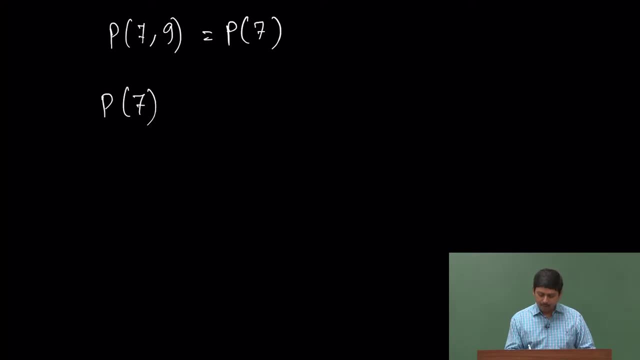 which is nothing but 7.. When you partition 7 into different parts, let us say I do this partition 5, 1, 1, 1, no 5, 1, 1, that is the partition which means that I have two particles in the level. 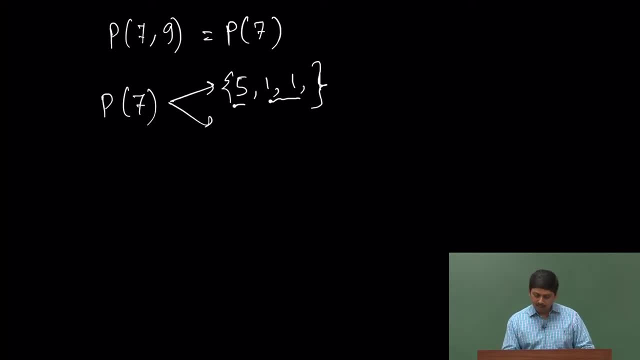 1 and I have one particle in 5.. So by now, let us say, I do one more: 4, 3,. 4, 2, 1, 1.. 4, 2, 1, 1.. 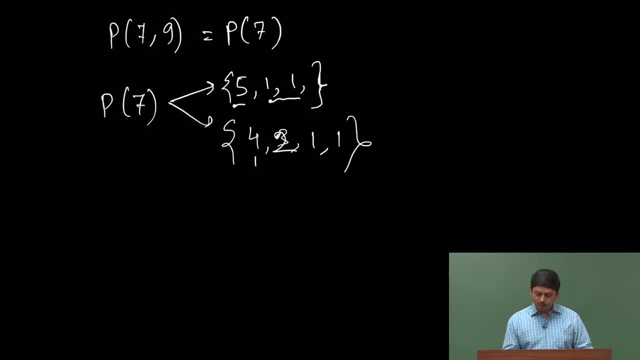 2, 1, 1,. this indicates that one particle having 4 energy, one particle having 2 energy and 2 particles are having 1 units of energy. so I am sorry, so we will just change that 4, 2, 1, 1 is like 8, so we will just do 4, 3, 2, 1, 1, 3, 2, 1, 1, so which means that: 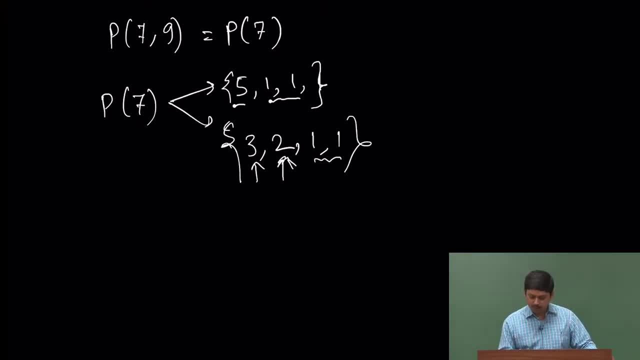 one particle is having 3 units of energy. one particle is having 2 units of energy and 2 particles having 1 units of energy. which means now, if I get all the partitions and count how many 1s are there, we will get number of particles corresponding to 1, 1 units. 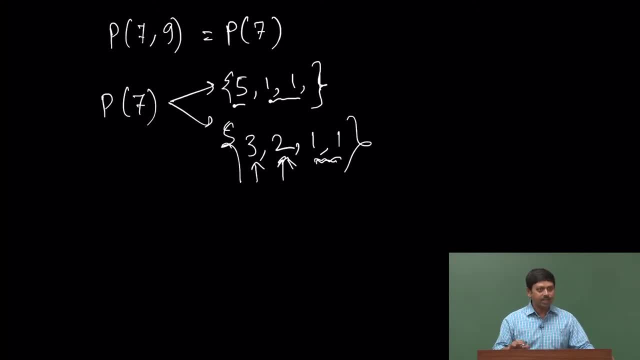 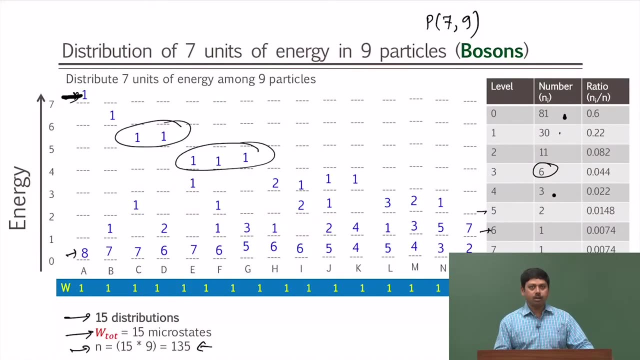 if we count how many 2s are there from all partitions, then we will get number of particles having energy: 2, like that we will get all possible values even without doing showing this particular distributions. we can use partitions to get that and by then we can. 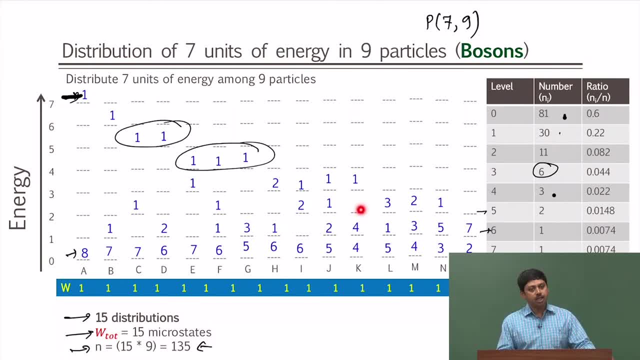 also count that how many particles are there, How many particles are there in which level. once we do that, we can just count them and divide by the total number of N and we get this probability distributions with energies. you see, this is my energy level and this is the probability we can plot, that which we 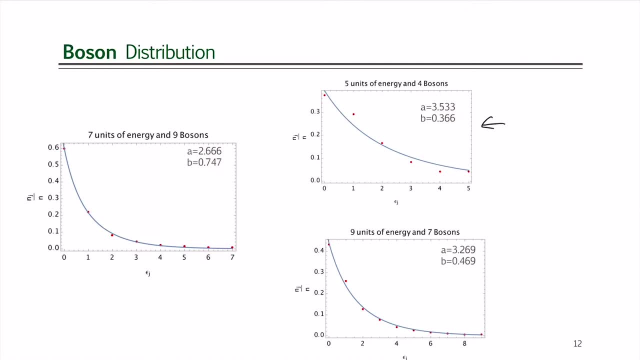 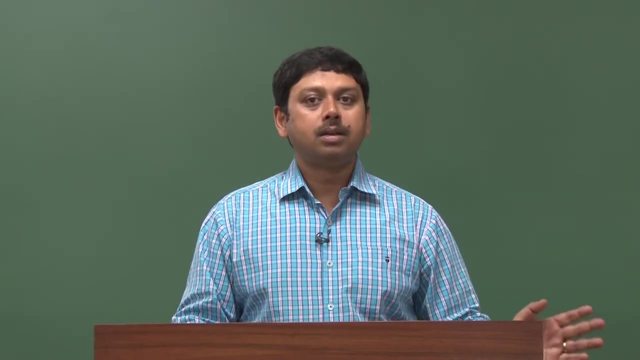 have done that. we have plotted that here for 5 units of energy and 4 bosons, 7 units of energy and 9 bosons and 9 units of energy And 7 bosons. but the fit is not an exponential fit, unlike the distinguishable classical particles. 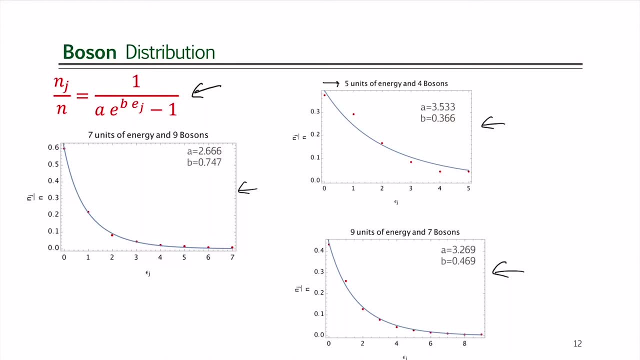 this fit is this equation. So what was the difference from the earlier one? if you see, the Maxwell-Boltzmann one was Ni by N was A, e to the power minus beta epsilon j. so if I write it differently it will become A by e to the power beta epsilon j. 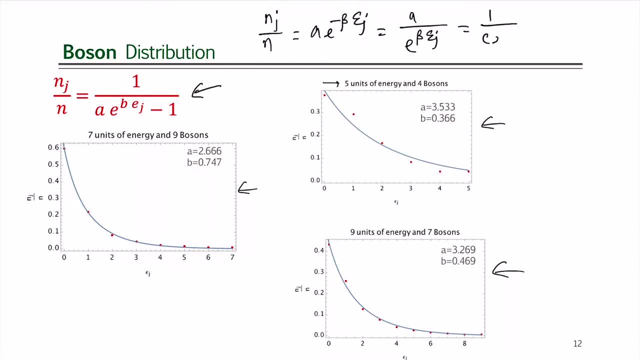 Or I can write it as: by bringing A down. I can write it as C, e to the power minus beta, epsilon j, You see here. or A prime, I can see instead of. so A prime is nothing but 1 by A. you see, the only difference is that there is a minus 1 in the denominator. this minus 1 was. 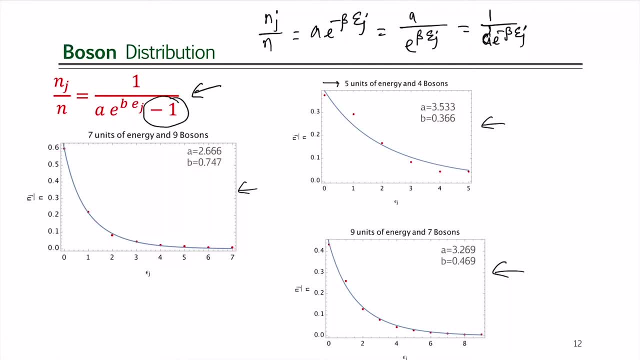 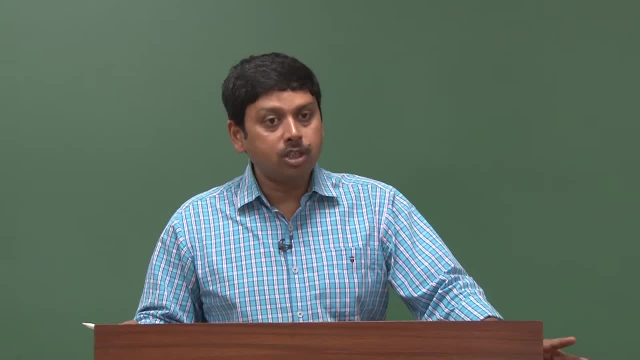 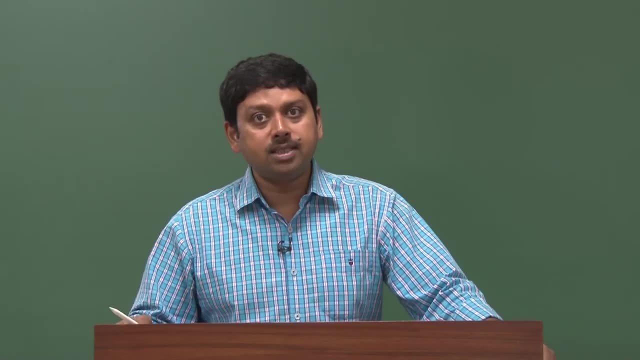 not there. in case of Maxwell-Boltzmann distribution, this minus 1 came because we are talking about now indistinguishable particles and especially bosons, because bosons do not have restrictions to B. many bosons can reside in the same level. that is an important characteristic apart. 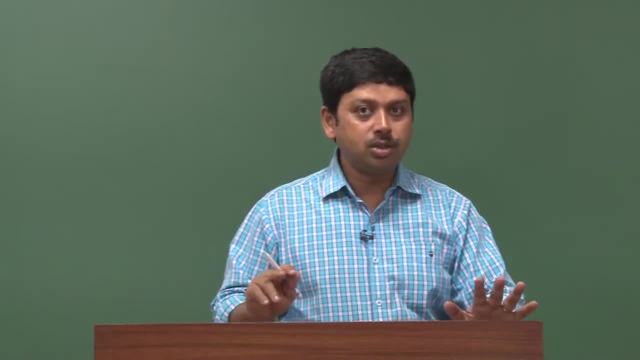 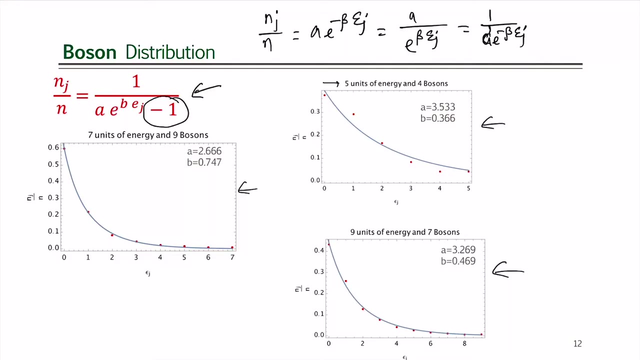 from being indistinguishable, These 2 characteristics, one is indistinguishability, another is many of them can reside, and that will give rise to this particular statistics. and I have fitted that with that particular line, although for 5, 4 it did not fit that well, but you see, it fitted really well for 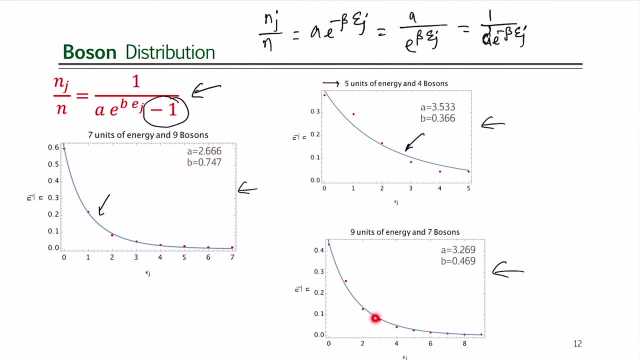 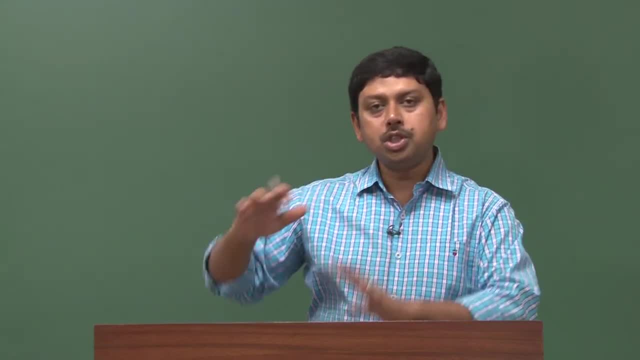 7 units of energy and 9 bosons, and also 9 units of energy and 7 bosons and it will fit very well when you increase the number of bosons. Ok, The number of particles. so you see that, going from distinguishable particles to indistinguishable, 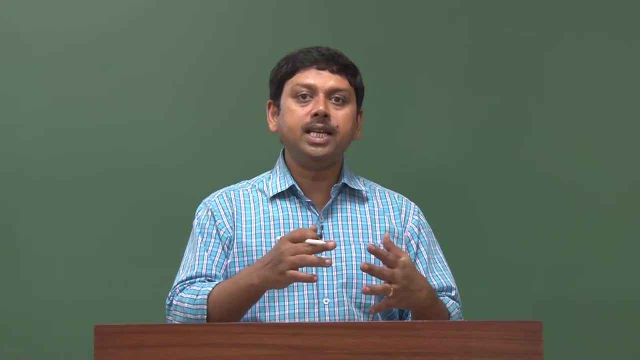 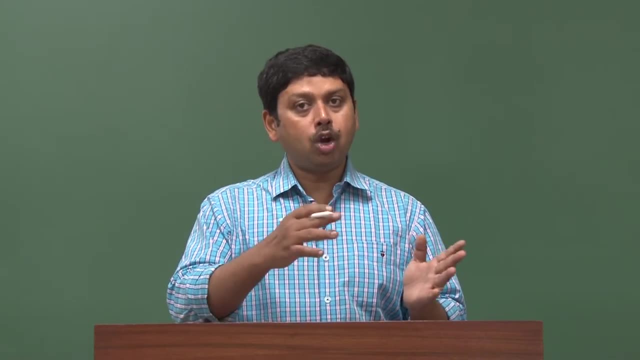 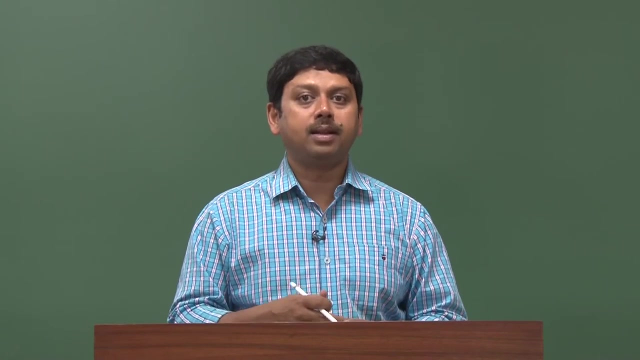 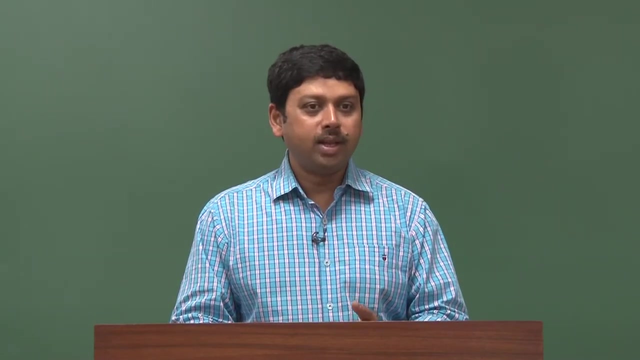 particles, your statistics. that means how the probability of occupying a particular energy level, how it has changed from a normal exponential distributions to something like this particular distributions, which is an experimental observations that it will. that distribution will follow this one. so now, if something follows this one, we know that. 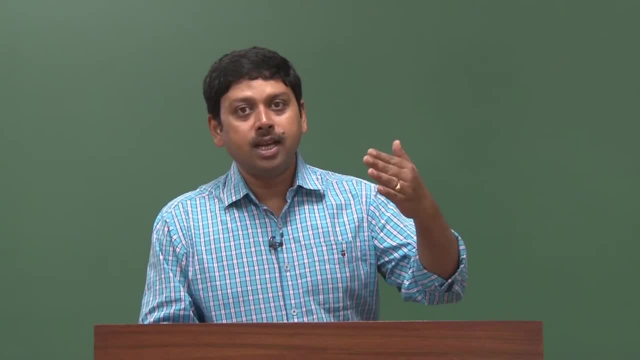 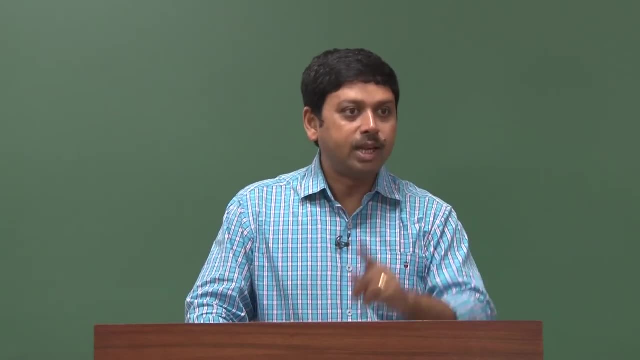 they are bosons, Whether we are able to distinguish or not. that is a secondary aspect. but if we get a statistics of particular distributions and it follows this one, then we know that. okay, we are talking about bosons, we are not talking about Maxwell-Boltzmann. 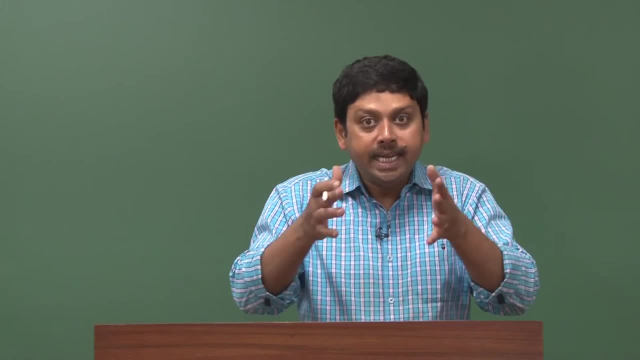 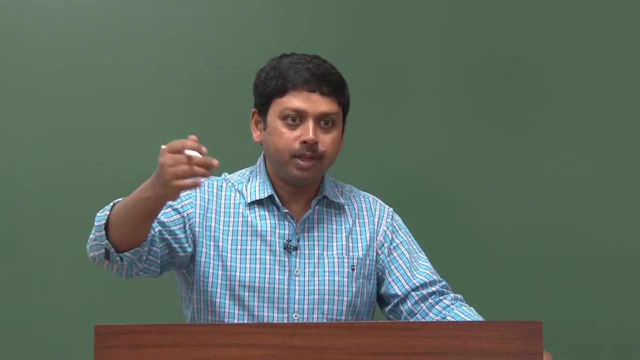 Now the fact that classical particles follow Maxwell-Boltzmann indicate that they are distinguishable, but our eyes cannot, may not be able to distinguish them. We see all, like you know, incense. let us say they look all the same colour we cannot distinguish. 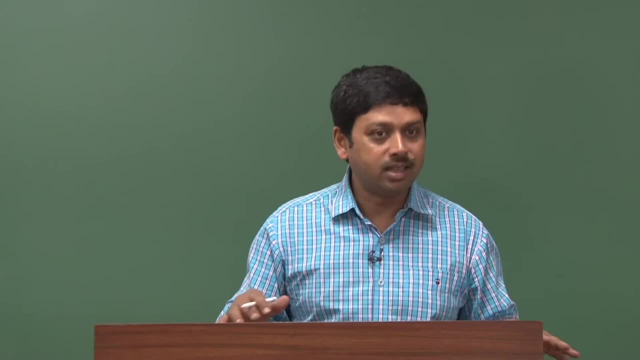 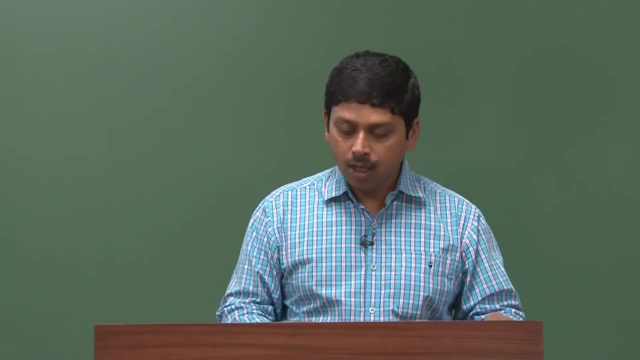 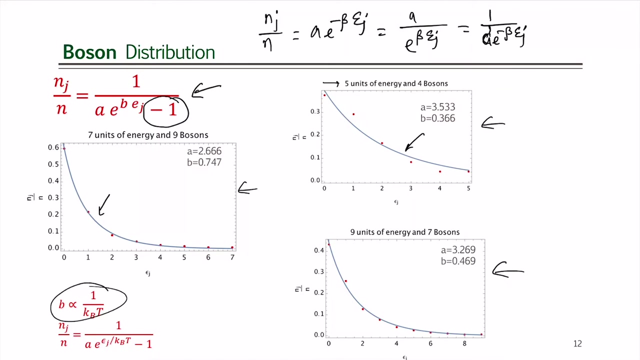 them, But our inability to distinguish or indistinguish has nothing to do with that. Whatever statistics we will get will tell us that what kind of particles we are dealing with. and that is the thing. So now we got bosons, and again B is nothing but 1 by KBT, which has a good implication. 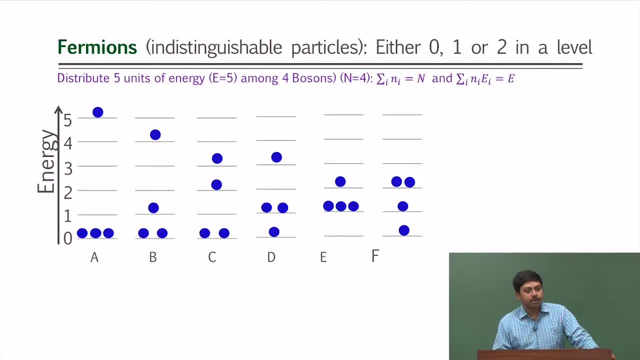 which we will talk about that later. Now let us talk about fermions. Now, what is the speciality Here? we are talking about same blue particles, except that since they are electrons or protons and they have, you know, half integer spin more than 2 cannot reside in the same level. 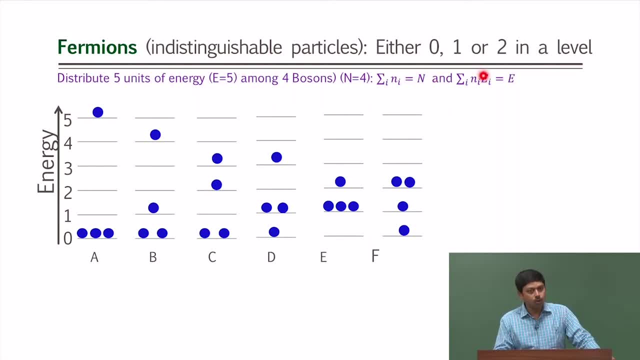 So the number of occupants, in any level, is 0,, 1 or 2.. Now we are talking about 5 units of energy and 4 fermions. this is fermions. So you see, since we are talking about 5 units of energy and 4 fermions, since we are talking 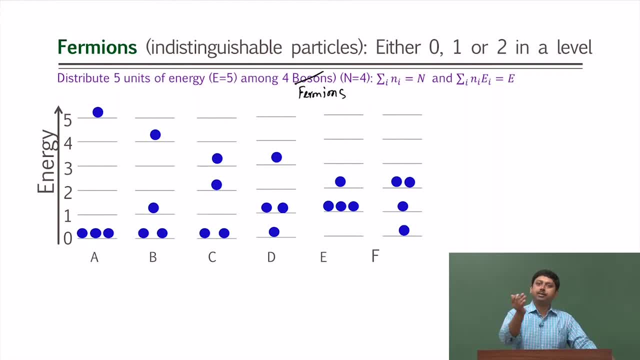 about 5-4 partitions. This is same as 5-4 partitions. This is same as 5-4 partitions as was there for other 2 particles also. It will be again 6 possible distributions. However, all 6 are not right for fermions. 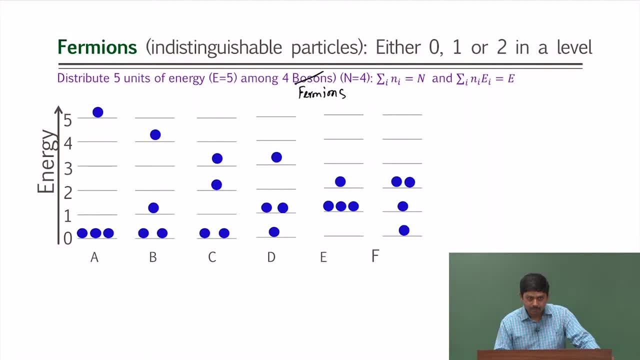 So can you tell me which one is not right? First one is not going to be right, because there are 3 particles in level 0. and which else is not right? Yes, that also will not be right, So we will end up not with 6.. 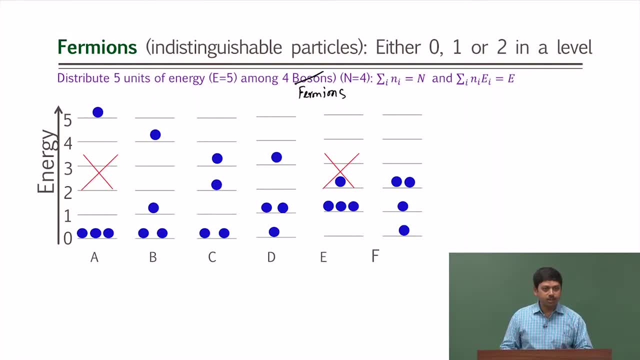 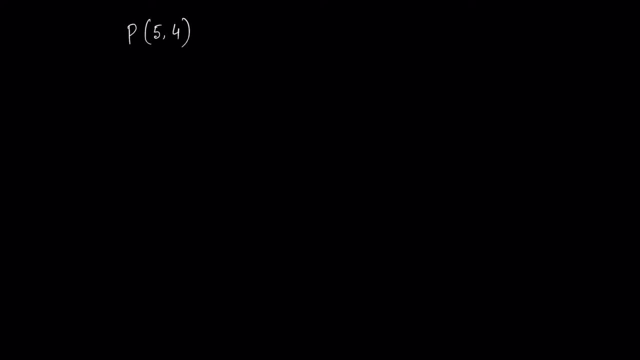 Because of that restriction, we will end up with 4 distributions. How do you get it? from partitions? Let us say you have 5 units of energy and 4 particles. Now you can partition the 5 units of energy among 4 particles in many different ways. 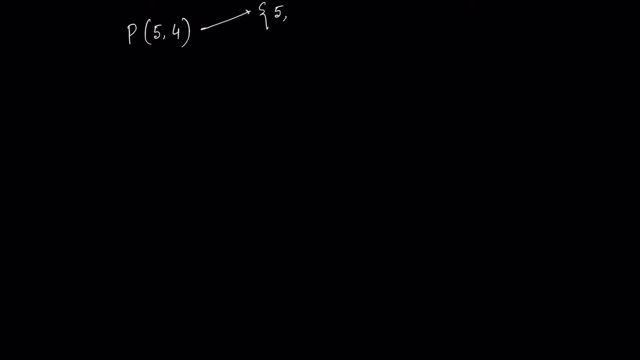 For example, you put 5 units of energy to 1 particle and then rest of the 3 particles get 0. Now this, according to the rules of the Pauli's exclusion principle, 3 particles will be in level 0 and therefore it will be not allowed. 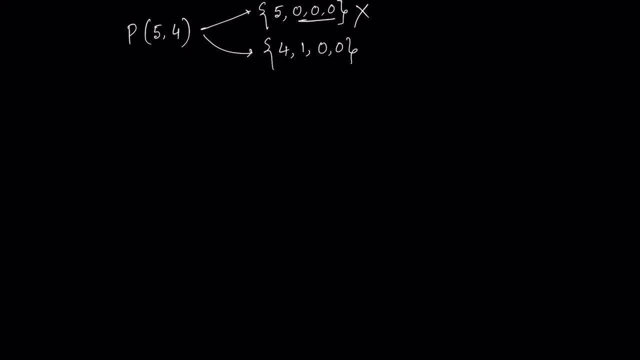 Similarly, you can break them into 4-1-0-0. that is an allowed one, because there are 2 particles only in level 0, 1 particle is in level 1 and 1 particle is in level 4.. Now, if you do 3-2-0-0, that is also allowed. if you do 2-2-1-0, that is also allowed. and 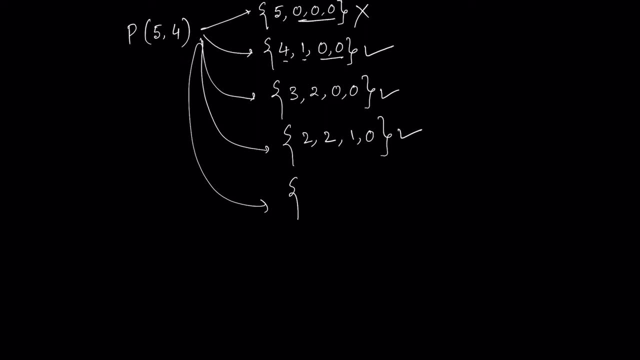 if you do, let us say 2-1-1-1, and that is not allowed transition, because there are 3 particles in level 1.. So for bosons, however, everything is allowed, because there can be more than 2 particles also in one level. so therefore, for fermions, you have to first see that. how many number? 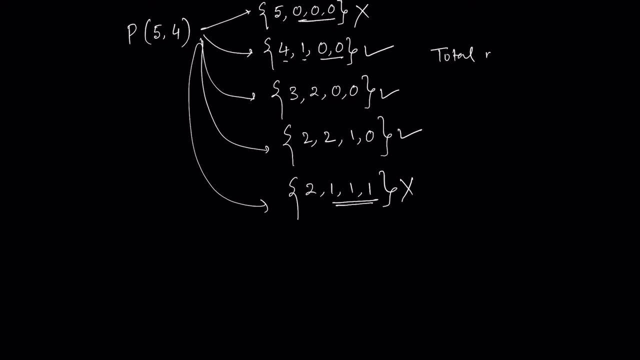 of distributions, Total number of distributions, and then from this total number of distributions you have to subtract the distributions in which more an integer number appearing more than twice Distributions where a particular integer. If you do that, then you will be able to get the number of fermions. 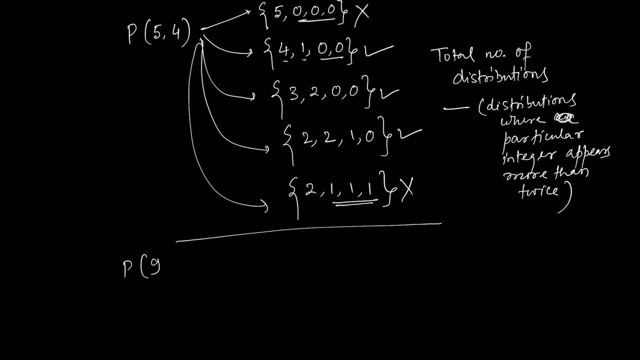 You can try that, for example, with 9 units of particle, 9 units of energy among 6 particles, and then you can have- let us say you can have- 9 and then 5 zeros. That will be enough. That will not be allowed. 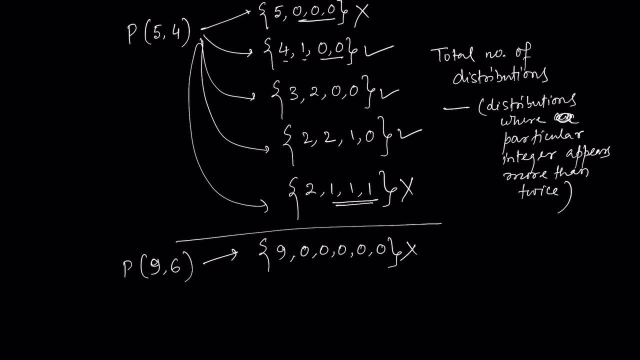 That will not be allowed. if you say 8-1-0-0-0-0, that is also not allowed- then you have 7-1-1-0-0-0, that is also not allowed. but then if you have, let us say, 5, then 2,, 5 and 2,, 7,, 7 plus 1,. 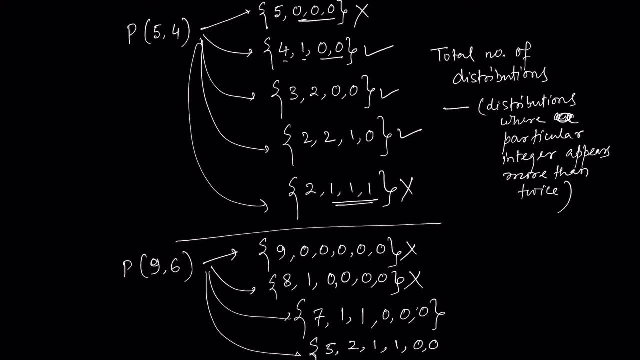 8 plus 1, 9 and 0 and 0. that is an allowed one, because the total energy is 5 plus 2, 7 plus 1, 8 plus 1, 9, 6 particles: 1,, 2, 3, 4,, 5, 6 and no integer is appearing more than. 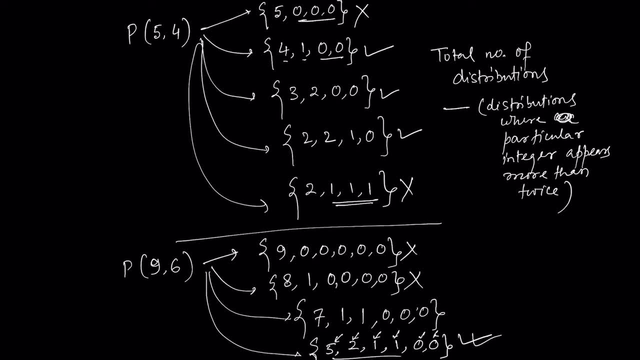 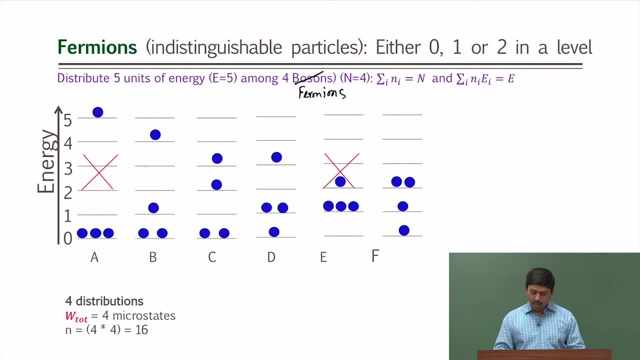 twice. So therefore, this is an allowed fermionic distribution where 9 units of energy distributed among 6 particles. So now you see, I am left with only 4 distributions, not 6.. So now you see, I am left with only 4 distributions, not 6.. 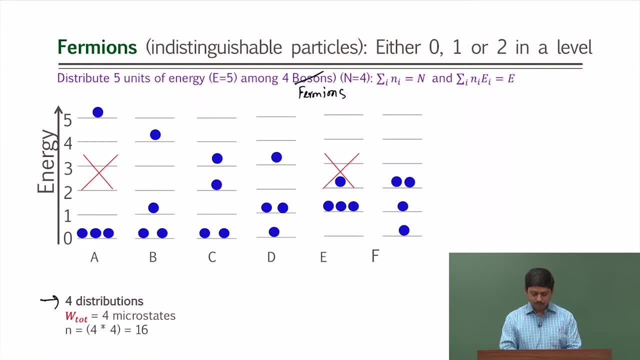 So now you see, I am left with only 4 distributions, not 6.. Only 4 distributions, That means total number of particles in 4 distributions will be 16.. Now let me count how many particles are there in which level. So, for example, level 5 has 0 particle because this distribution was not allowed. 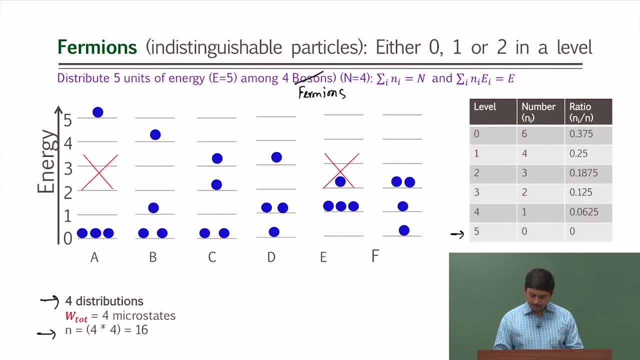 So nothing can go to level 5.. Level 4 has 1 particle which is coming from this distribution B. Level 3 has 2 particle coming from this And this distribution. Level 2 has 3 particle coming from this one and this one. 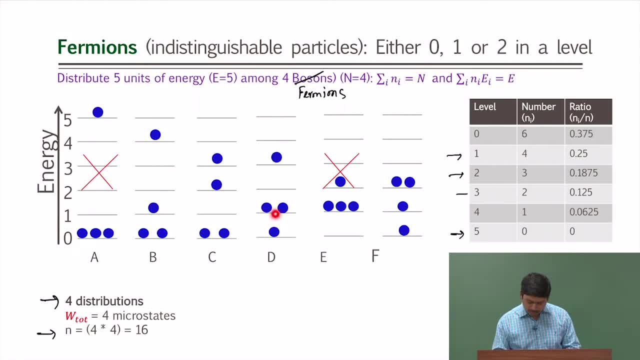 Level 1 has 4 particle coming from this one, this one and this one, And level 0 has 6 particle, as you can see, not coming from here, but 2 plus 2 is 4,, 5 and 6.. So once we get that, I divide 6 by 16, I get this number. 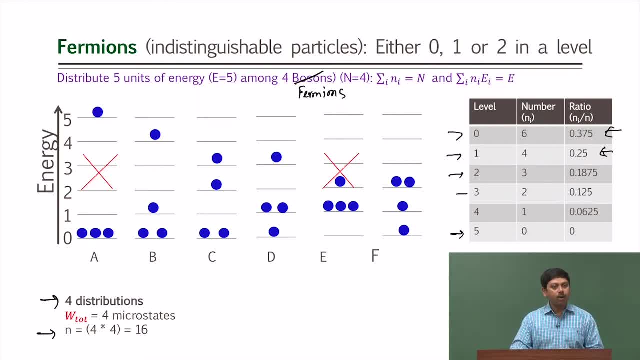 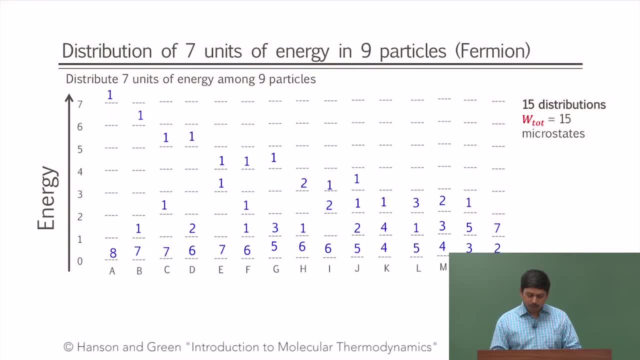 I get, divide 4 by 16, I get this number. So I get now again the probability with the energy level. So I get now again the probability with the energy level. Similarly, can you tell me which distribution? So again, I am now dividing 7 units of energy among 9 particles, and I got the same I wrote. 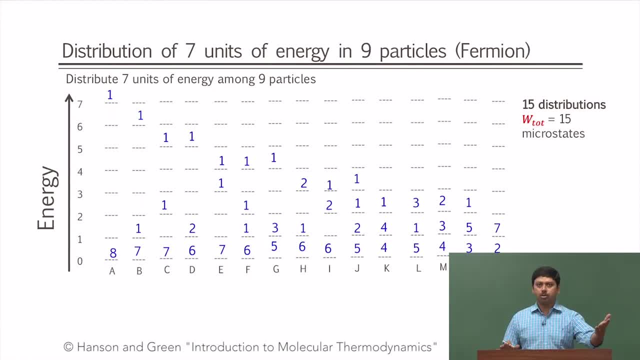 down the same distribution as was in Bosons and Maxwell-Boltzmann distribution. Now, which of them is allowed, can you tell me? Actually, none of them is allowed, because in every distribution there is one level which has more than 2 particle. For example, here 8 is more than 2, here 7 is more than 2, 7 is more than 2,, 6 is more. 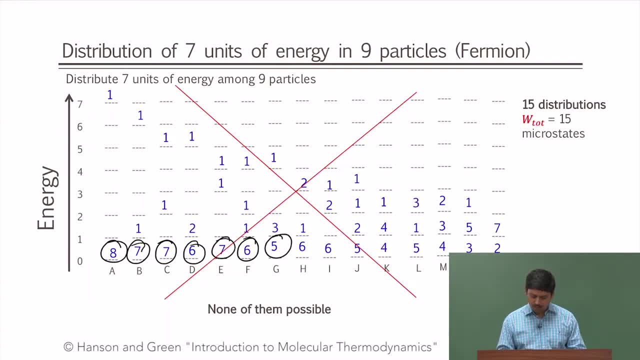 than 2,, 7 is more than 2,, 6 is more than 2,, 5 is more than 2. of course, 6,, 6,, 5,, 4,, 5,, 4,, 3 and here 7.. 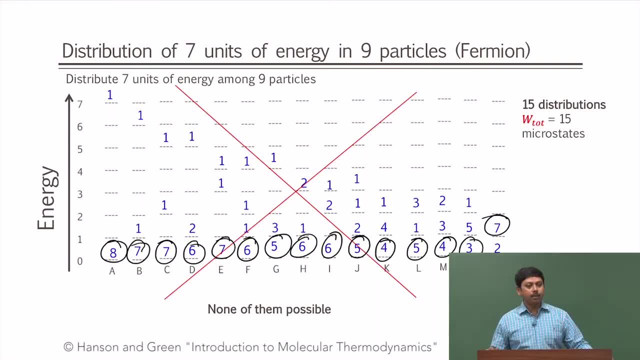 So I do not find any in which the number of particles is in every level is 2 or less. So 7 units of energy cannot be distributed in 9 particles for fermions. So for fermions your energy level should be more than the number of particles. 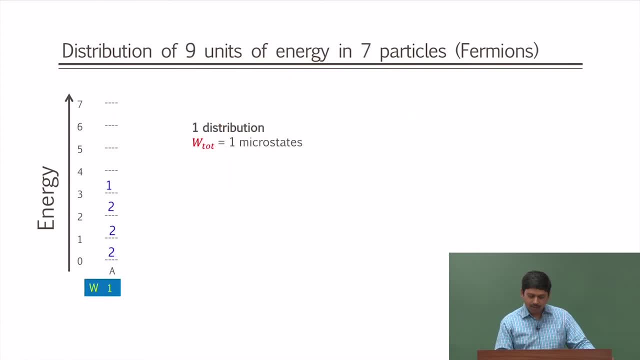 So let us switch it around. let us do it: 9 units of energy in 7 particle, and you can see that there is only one possibility. You cannot change it to anything else. only one distribution, only one microstate. if you have 9 units of energy and 7 particles for fermions. 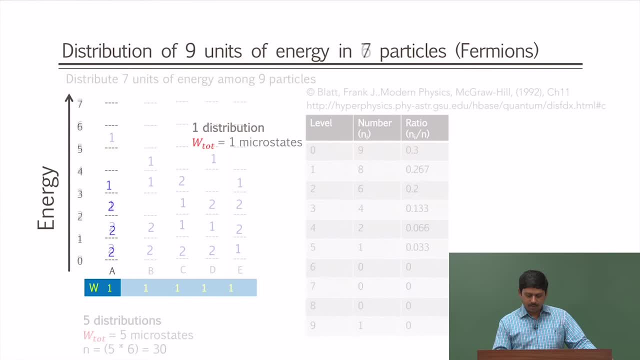 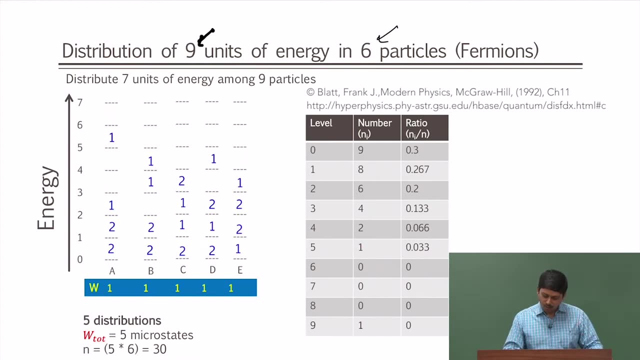 Now, if I reduce the number of particles, if I reduce the number of particles, if I reduce one particle- 9 units of energy, into 6 particle, I get this many possible distributions: 1,, 2,, 3,, 4,, 5 distributions I get. 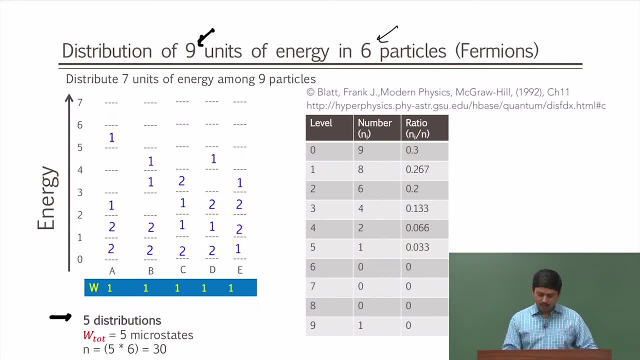 So now for 5 distribution. I have total number of there are 6 particles, so I have total 30 particles and I can count that how many levels, at which particle, As you can see that 6,, 7,, 8,, 9 will have 0 particle. 5 has only 1 particle, 4 has 0,. 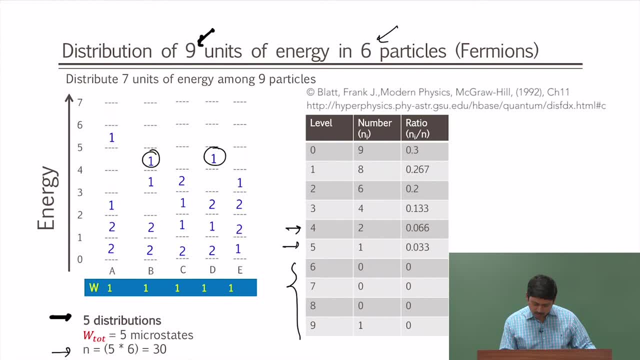 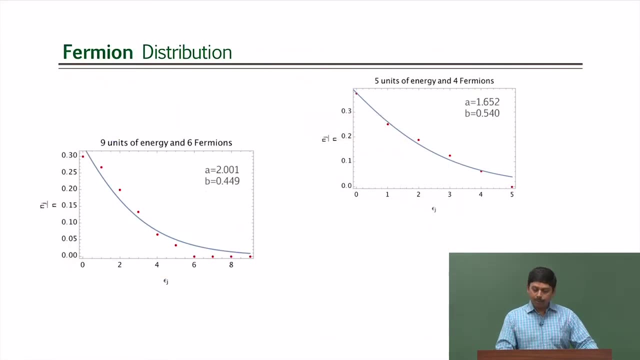 3 has 2 particle, 3 has 4 particle, 2 has 6 particle and 1 has 8 and 0 has 9 particle and corresponding probabilities are given here. So we have plotted 5 units of energy into 4 fermions and 9 units of energy into 6 fermions. 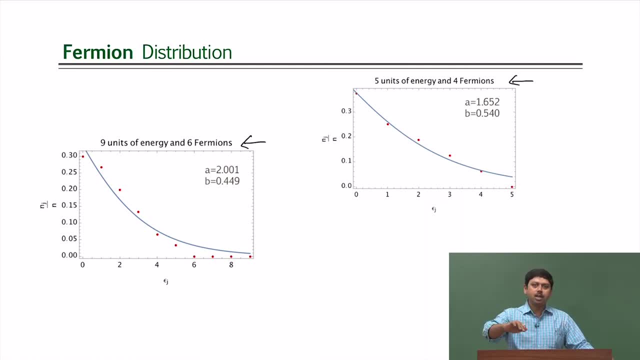 because the other 2 are not possible. 9 units of energy in 7 fermions gave us only one distribution, which is statistically impossible, Statistically not good, and 7 units of energy, 9 particles, did not give us anything. So we just landed up with these 2 and we have shown you. but, however, in this case the fitting 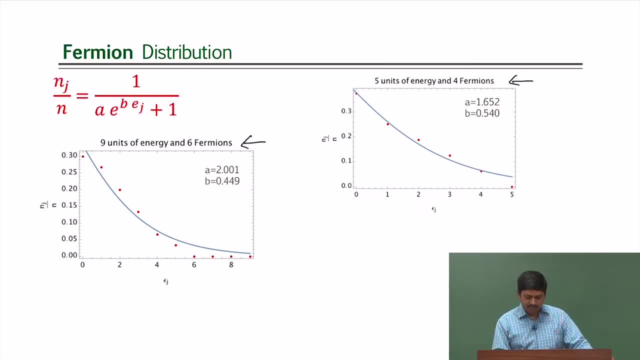 is not by any of the other 2 equations. the fitting is done by this equation. So remember, for bosons it was minus, for bosons it was minus. and for Maxwell distribution there was for Maxwell distribution this plus 1 or minus 1 was not there, okay.